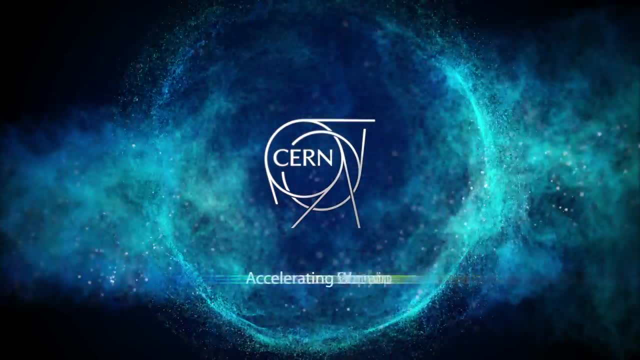 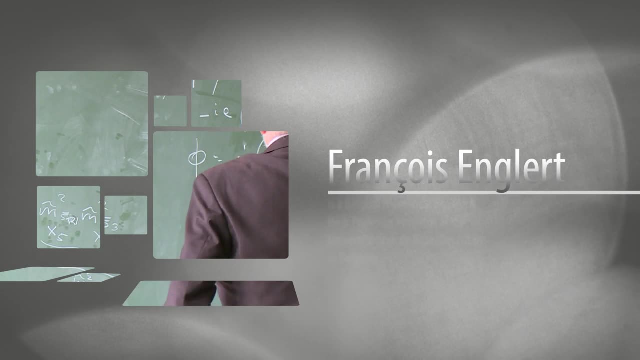 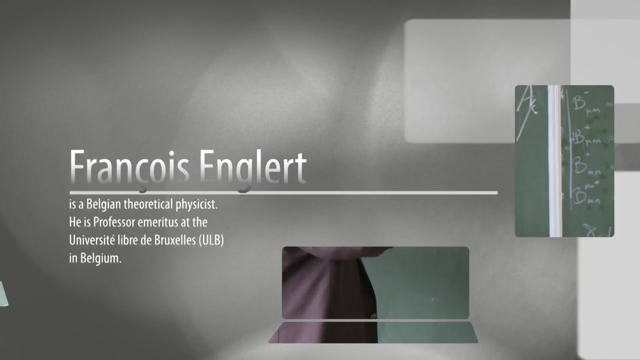 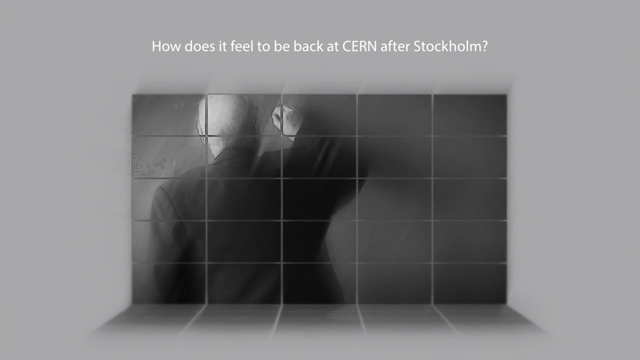 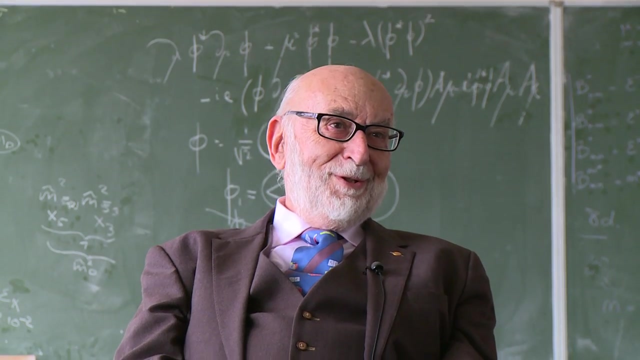 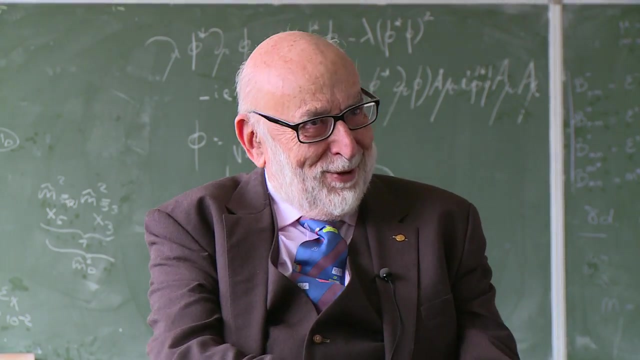 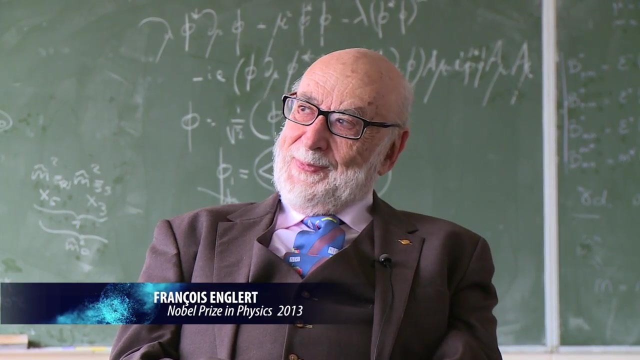 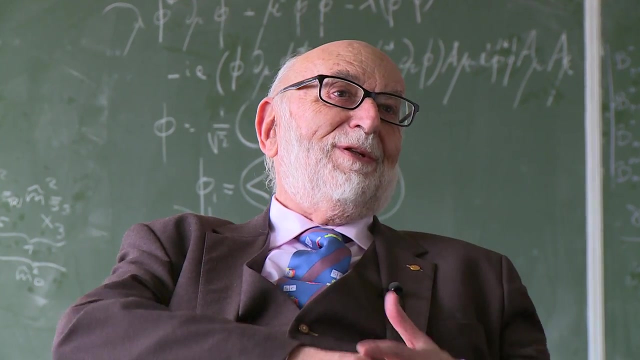 Thank you for watching. I'm a little bit tired, But that doesn't mean I don't feel well. I feel well after Stockholm, of course, But yeah, so it's well. in a sense, it's very nice to see that this thing has developed the way it should. 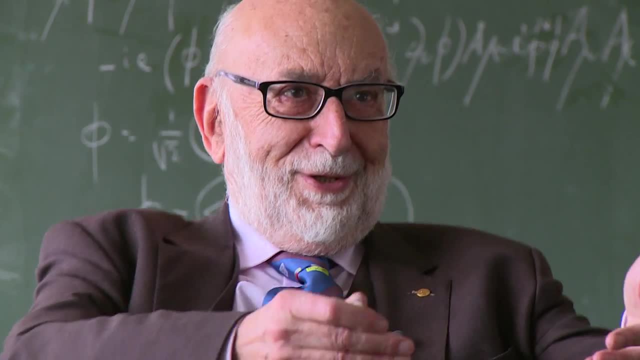 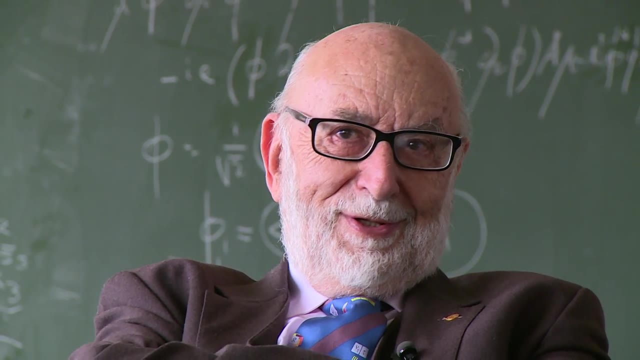 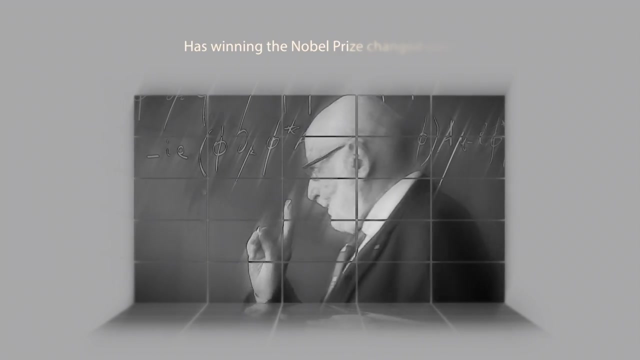 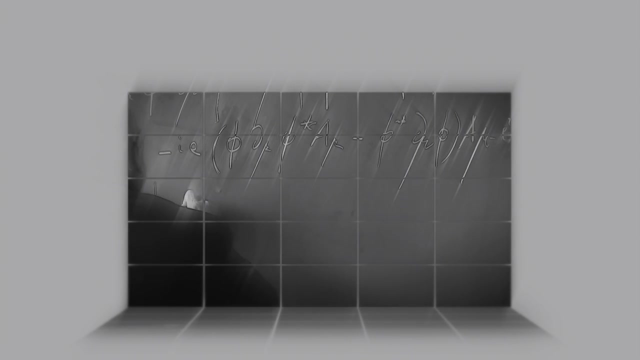 And I mean the particle, I don't mean me, And I think this is really a great discovery And I'm very happy, of course, to have it at all the price. Well, it's trying to change me. I don't, you know. for the most part, it's trying to change me. 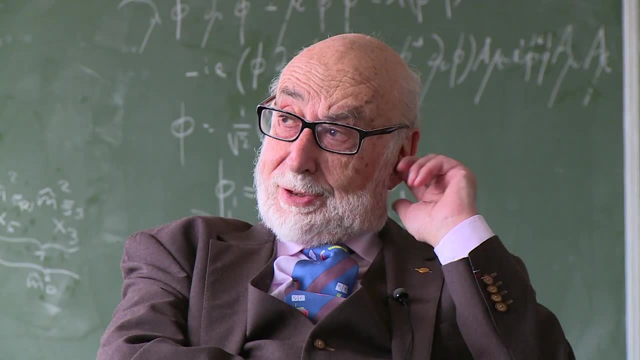 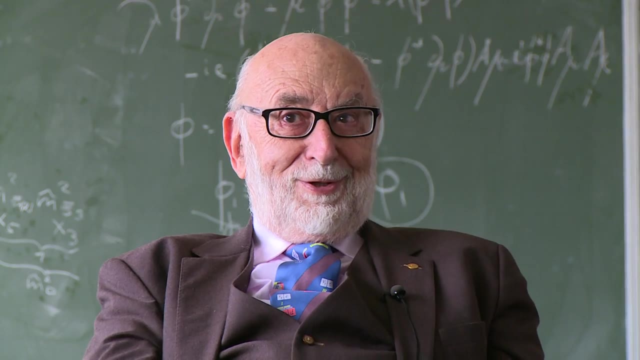 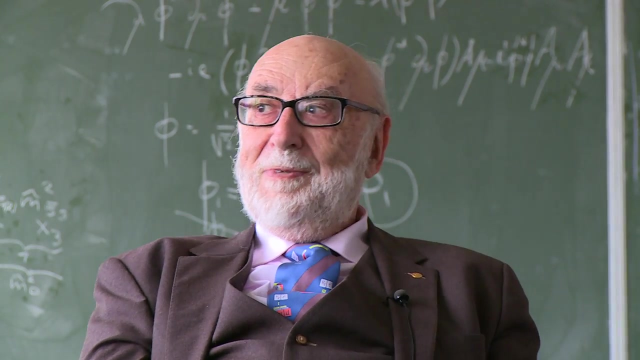 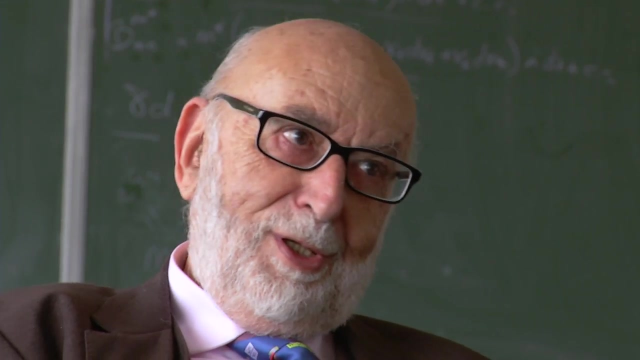 It has such a large spectrum of people who are interested in this that in a sense I'm a little bit shocked, But at the same time I think it's not so bad, because it really spread the interest in something that people generally don't show so much interest, which is actually fundamental to science. 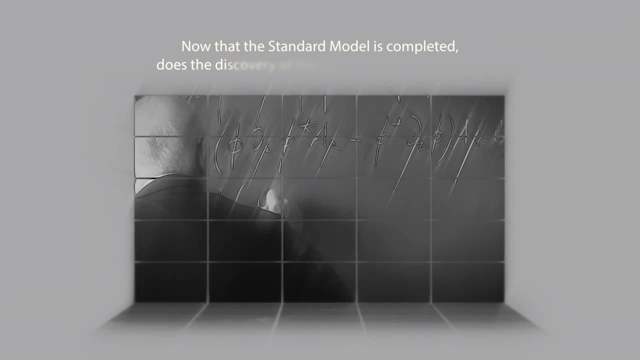 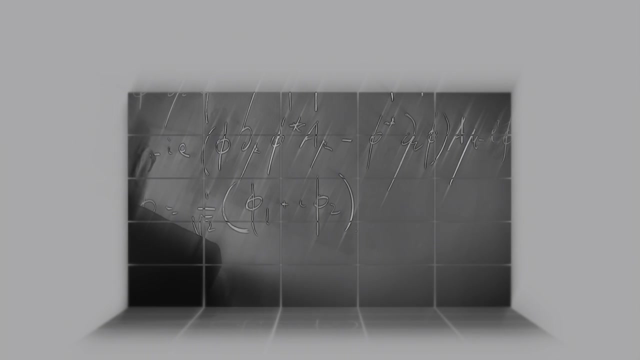 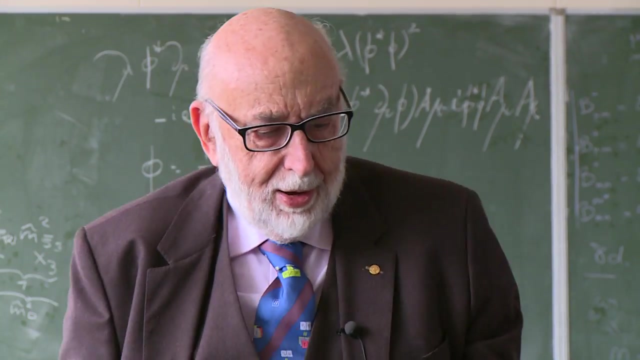 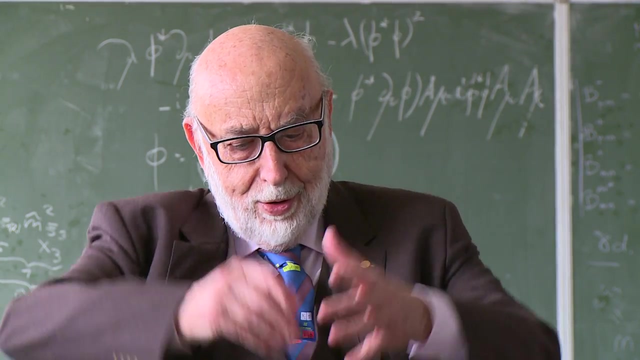 Yes, I think it does. The point is this: You could have imagined that when you discovered this particle, let's call it the scalar boson or the Higgs boson or the pH boson, whatever name- scalar boson is the physical name. 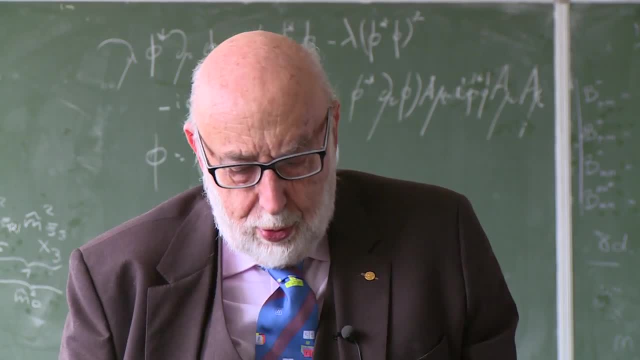 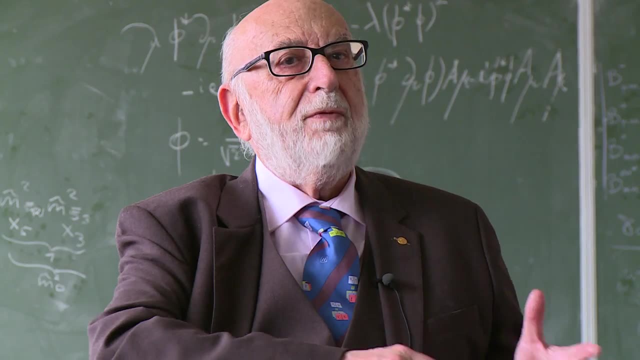 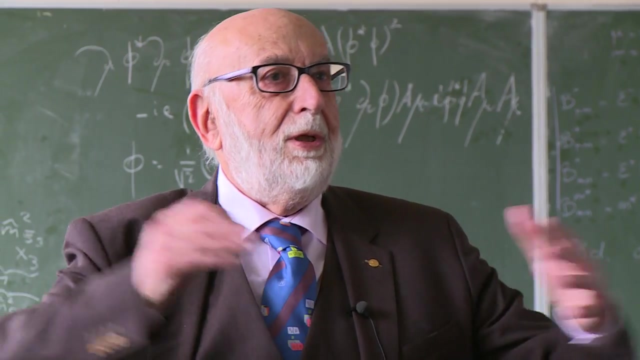 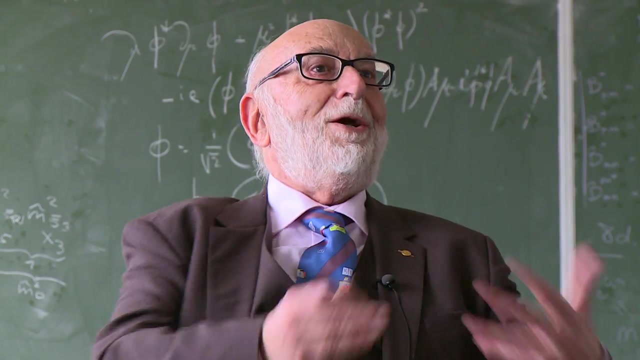 And when you discovered this, you could have imagined that you would also have discovered in the neighborhood all kinds of other particles. Now, some people were unhappy that you didn't, that you just found this. I found this is extremely interesting and it's probably the greatest part of the CERN discovery that nothing was around at that level. 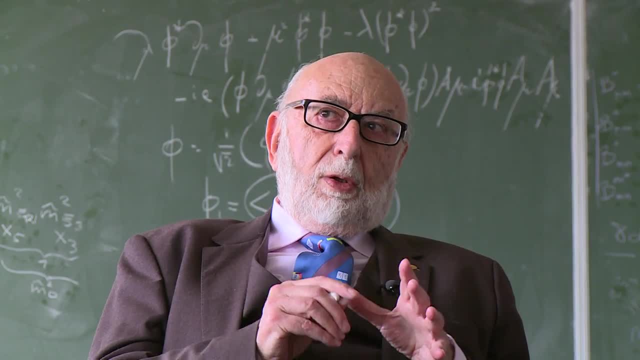 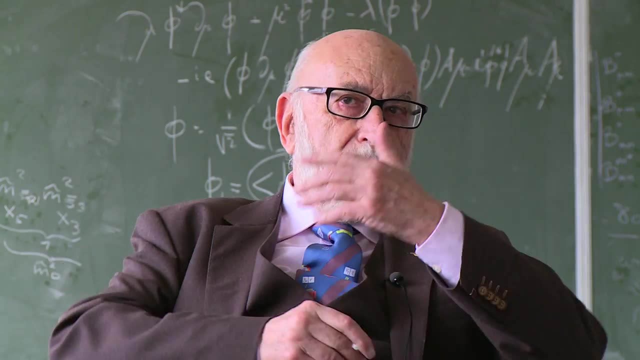 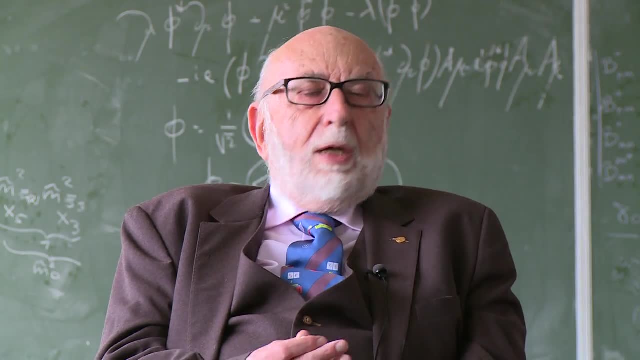 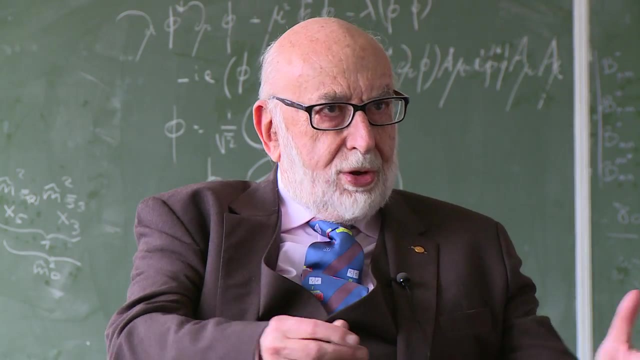 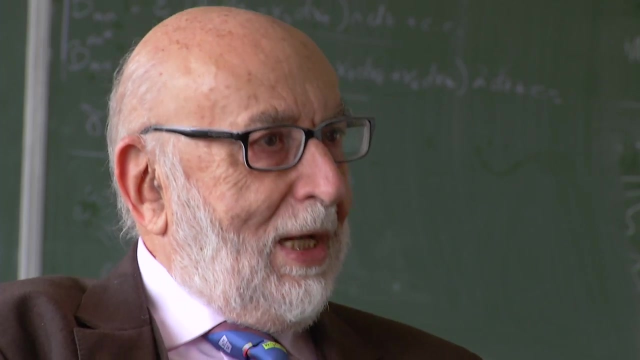 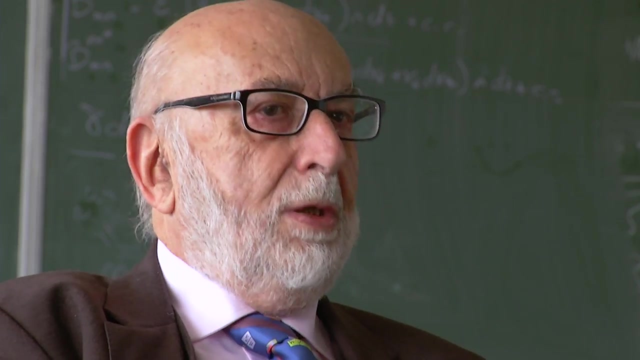 just sketched here are essentially not right. In other words, these fields behave at these energies like any elementary particle, Call it the electron or call it the quark, But that behaves essentially the same way, except that it is what I say, scalar, meaning that it's spin, a quantum property that describe, if you wish, its rotation. 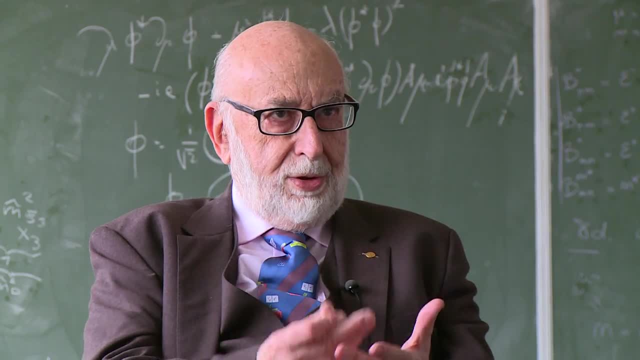 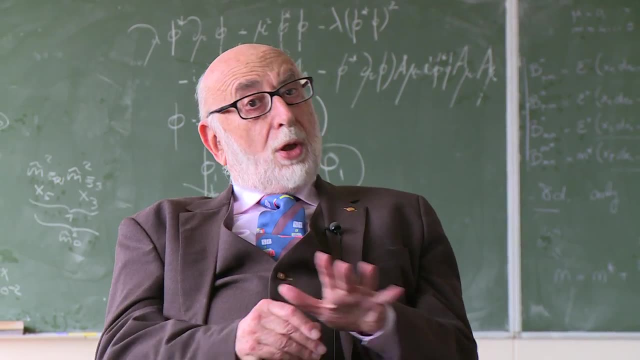 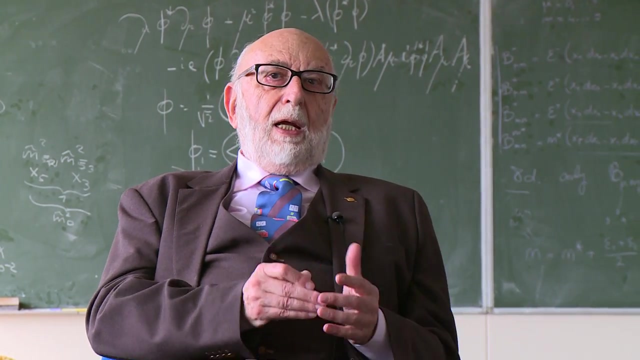 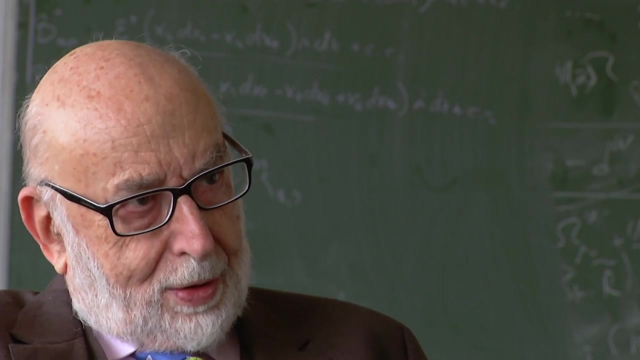 around itself that that is zero. This is a particle which does not define any orientation or axis of rotation or anything. So that means that that particle is, at that level, elementary, And that is extremely important because not only it closes the standard model, which is 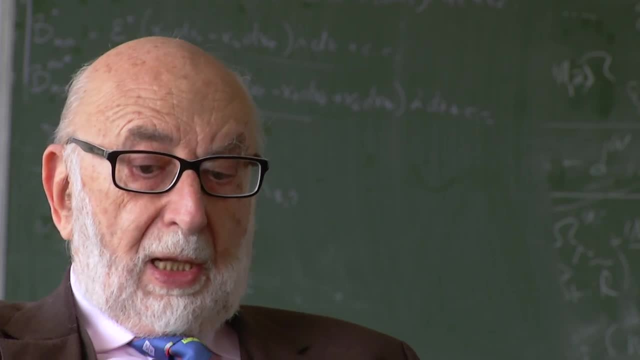 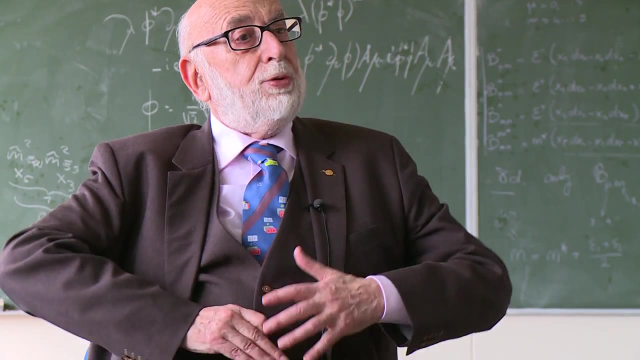 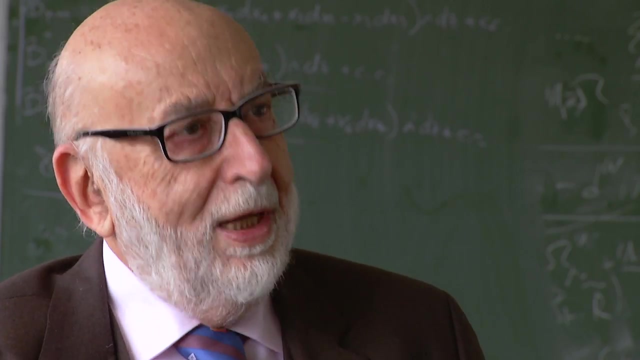 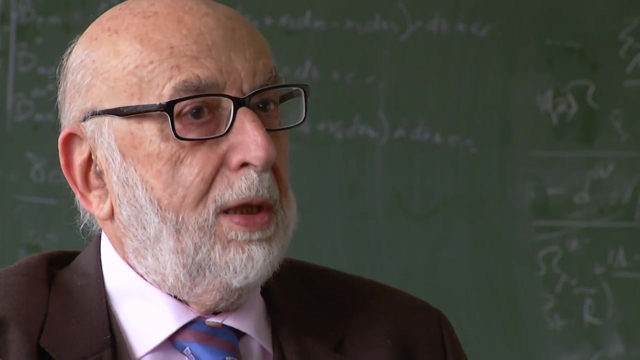 our present understanding of the particle we know, but it also indicates that whatever exists which we have not yet discovered, is probably much simpler than what would have been if we would have found a lot of particles around, which would mean that this particle here is essentially a composite of a lot of other things.